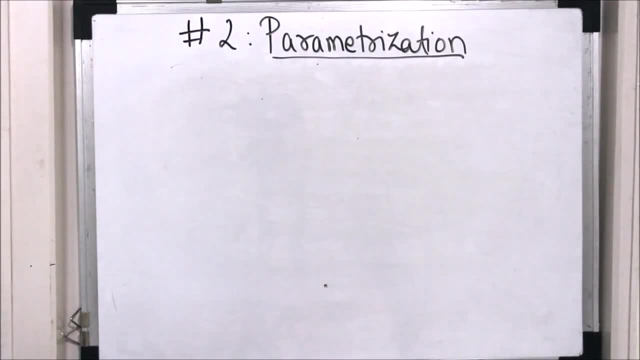 Hello everyone. so welcome to the second session, which is on parameterization of a curve. So today we will see how to parameterize a curve and after that we will go to the definition of an integral. So when you say a curve is a parameterized curve, 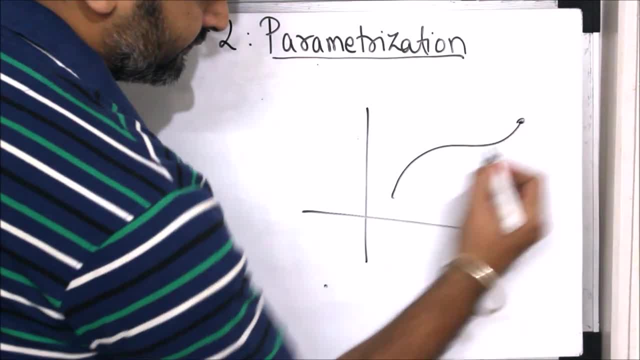 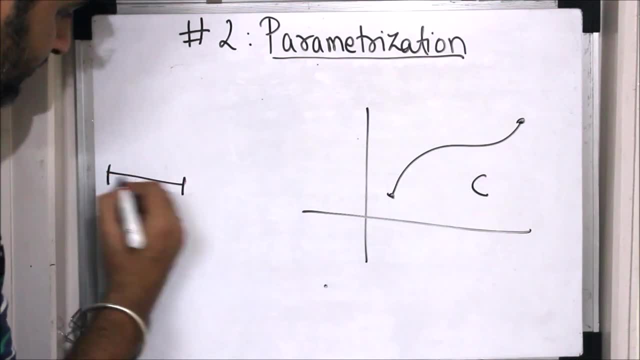 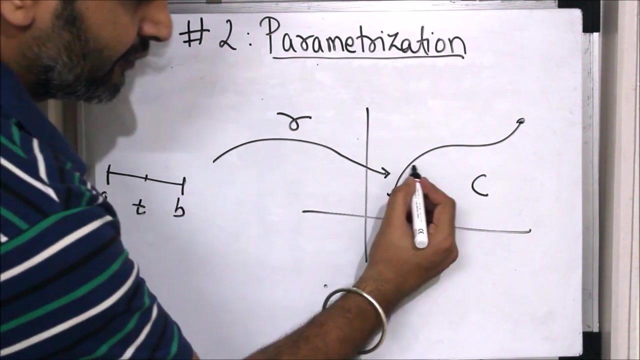 So suppose, if you have a curve and when you say this is a parameterized curve, if you are able to define a function r such that this is a subset of real numbers. So if I am able to define a function such that if I take any t over here, its image is what This point on the curve. 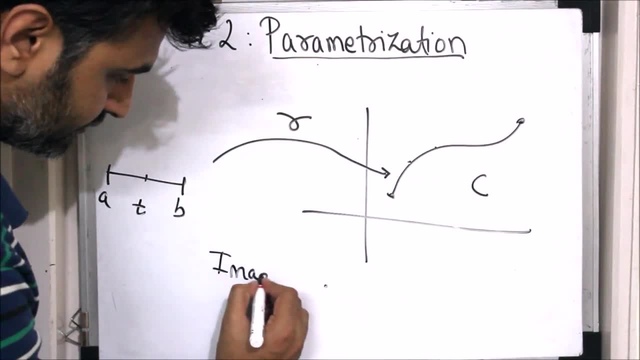 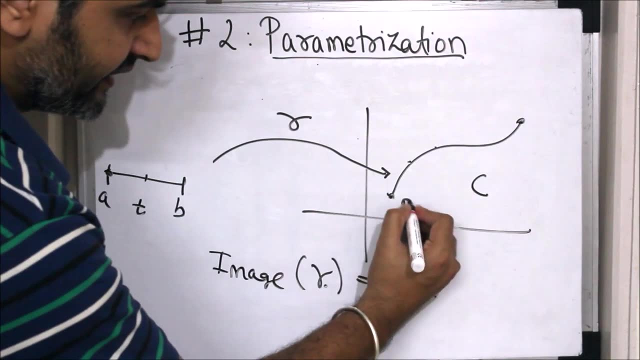 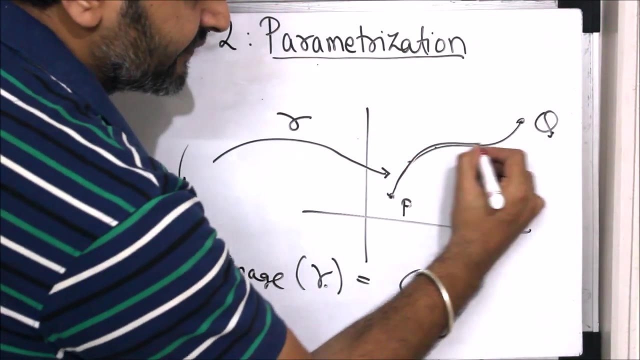 So if the image of this function is the curve c, that means a will go to what This point say p. Suppose your b, it will go to say q and as you go from a to b you get all the points from p to q. 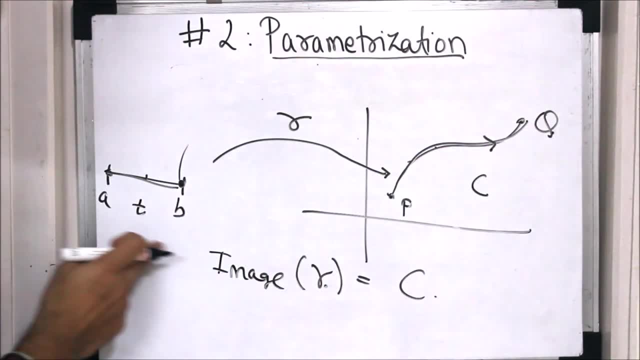 So if you get all the points from p to q as you travel from a to b, then I will call such a curve to be a parameterized curve. So what is a parameterization? So, if you are able to define a function from a subset of real numbers to the curve, such that the image of that function is the given curve. 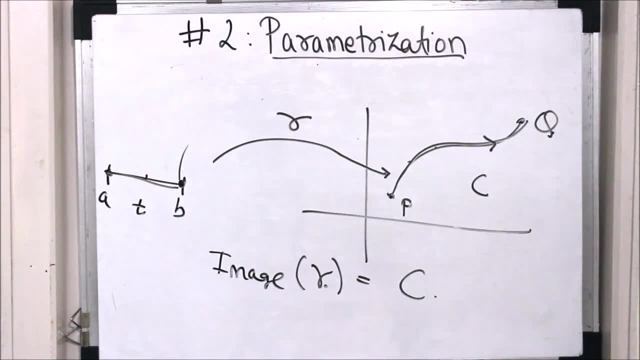 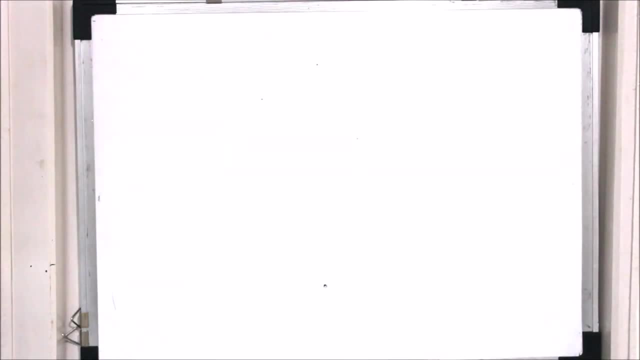 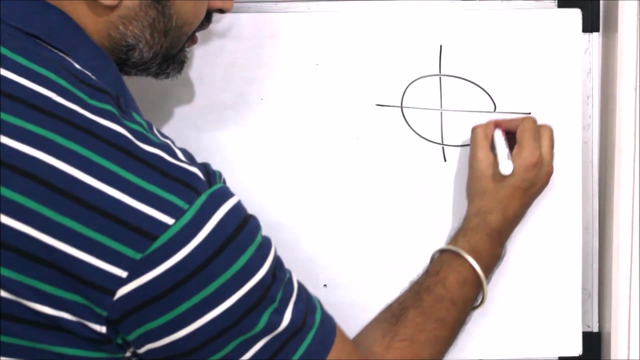 Then such a thing is called a parameterization, Or such a curve is called as a parameterized curve. So let me take some examples. Let's start with the standard examples. So suppose if I take circle, Suppose if I want to parameterize a circle of radius 2.. 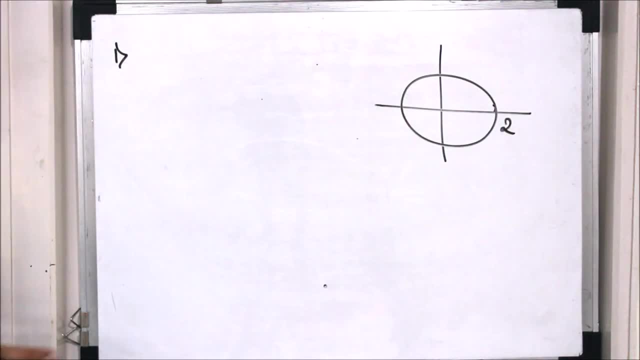 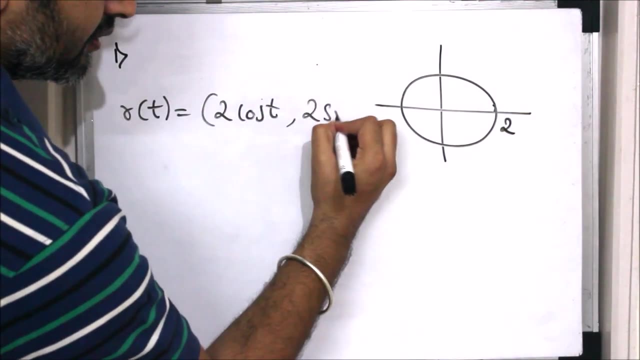 So we know that the standard parameterization of a circle is what? So if I define r as 2 cos t, 2 sin t, Where my t is what? 0 less equal to t, less equal to 2pi. 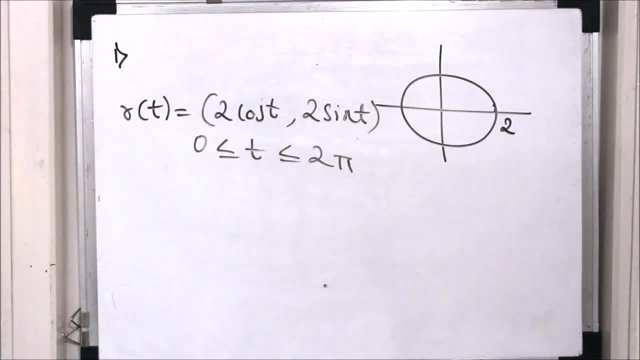 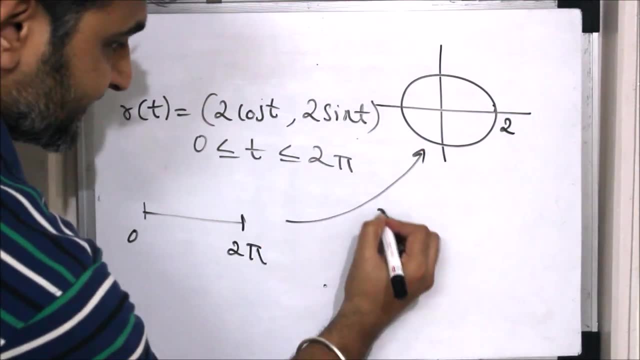 So if I define this as my function r, What is r? It is a function from this interval. What is the interval? 0, 2pi to this? This is my r. So if you see where your 0 will go, 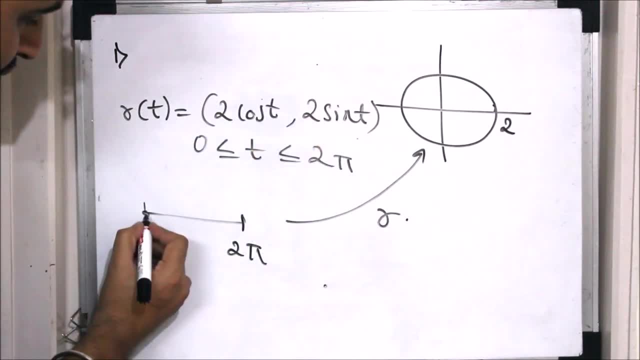 Your 0 will go to 2, 0.. So your 0 will go to 2, 0.. If I take pi by 2.. Where my pi by 2 will go, cos pi by 2 is 1.. 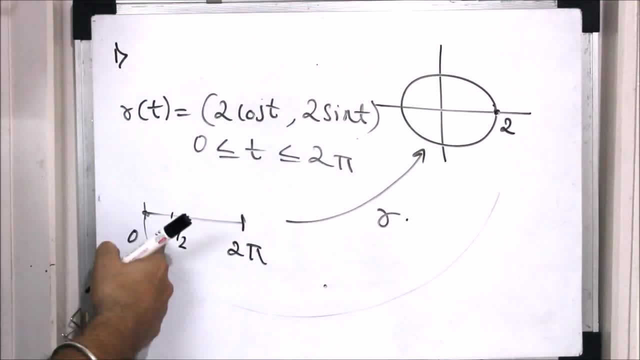 sin pi by 2 is 0.. Sorry, cos pi by 2 is 0.. sin pi by 2 is 1.. So pi by 2 will go to 0, 2.. So, in short, as you go from 0 to 2pi. 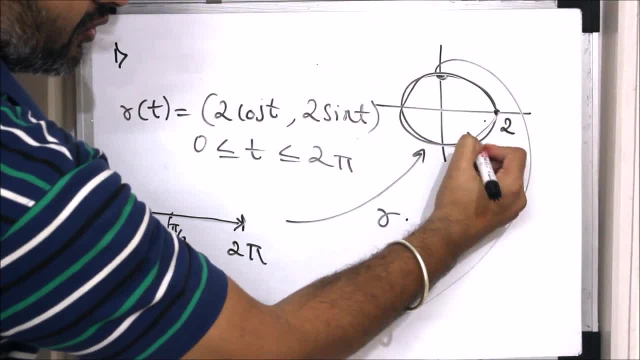 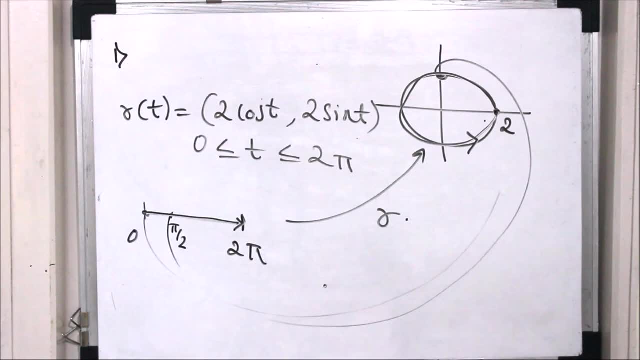 You get all the points on this circle of radius 2.. So this is what the parameterization of a circle is. Therefore, a circle is a parameterized curve. Here my radius was 2.. If my radius is some r, Or if my radius is some, say a. 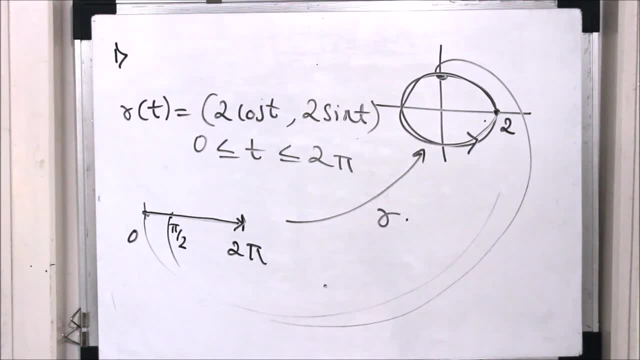 Then it will be a cos t, comma, a sin t. So that is the parameterization of a circle. And suppose: if you don't want whole circle, Suppose if you want only upper half part of the circle, Suppose if you only want this, much of the curve. 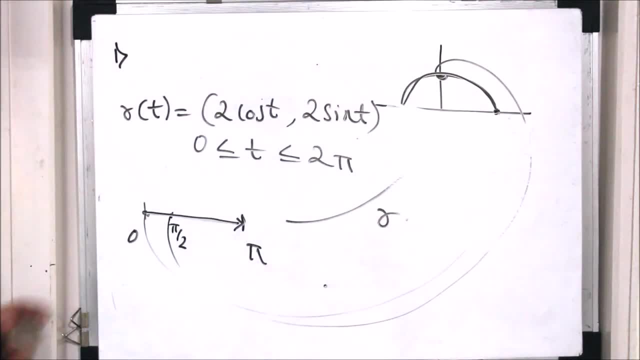 Then what will be my domain? My domain will be 0 to pi. So if I take from 0 to pi And I get the same function, I will get the upper half of the curve. Similarly, whatever part you want. 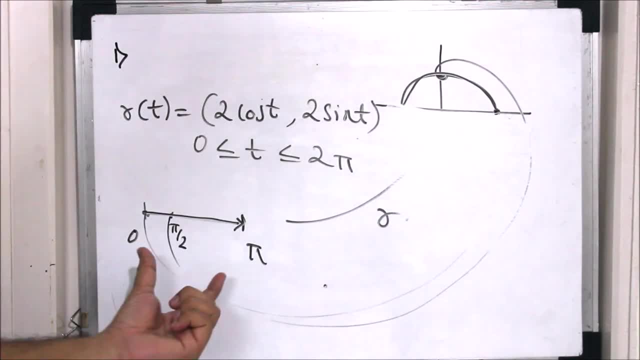 What you do is you simply keep on changing this domain. You keep on changing this domain, You get the respect to arc of that circle. So that's how you get whole of circle. And suppose, as you can see, The circle which I drew just now, 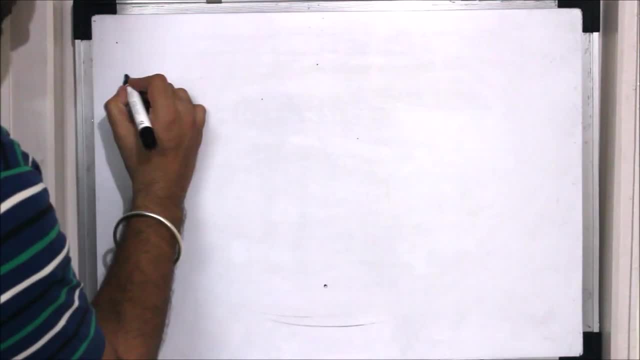 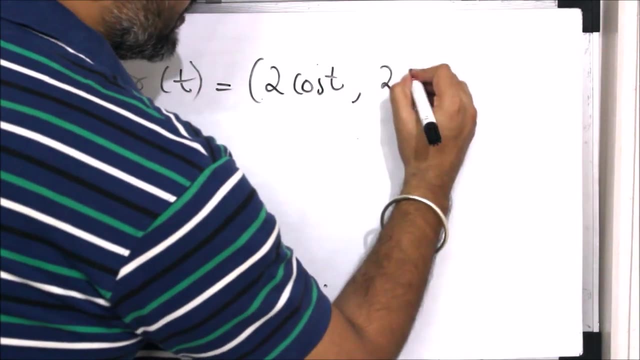 It was a circle in xy plane. So it was a circle in xy plane. So suppose, if you are in a space, So what I will do, I will write this as 2 cos t comma, 2 sin t comma 0.. 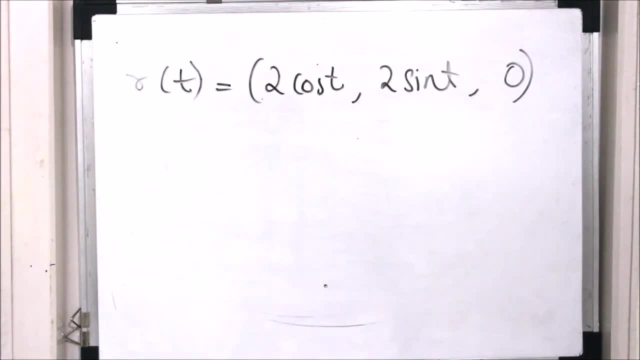 To stress that in R3. I am looking at the circle with center 0, comma 0 and radius 2. And that circle is in xy plane. That means my z is 0. But suppose if you have x equal to minus 2 plane. 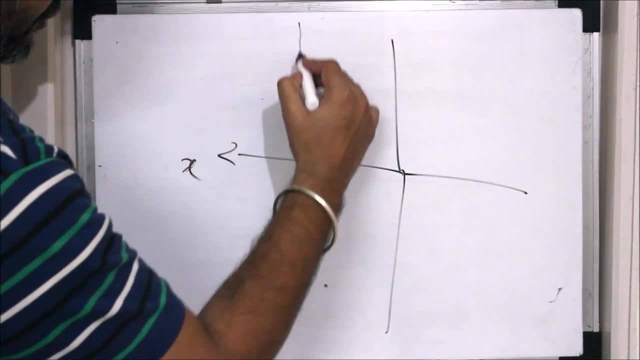 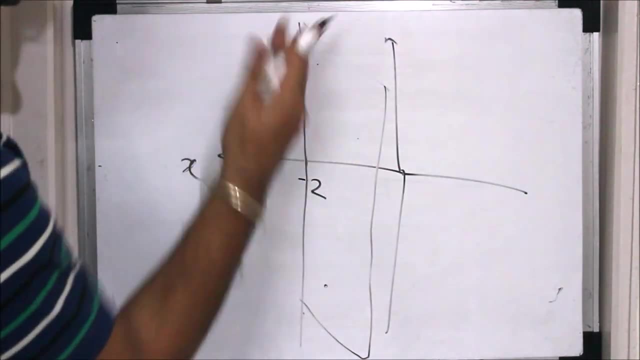 Suppose this was x equal to minus 2.. So like you have a plane over here, So you have this x equal to minus 2 plane, So this is the plane, So this is the plane over here And you have a circle in this plane. 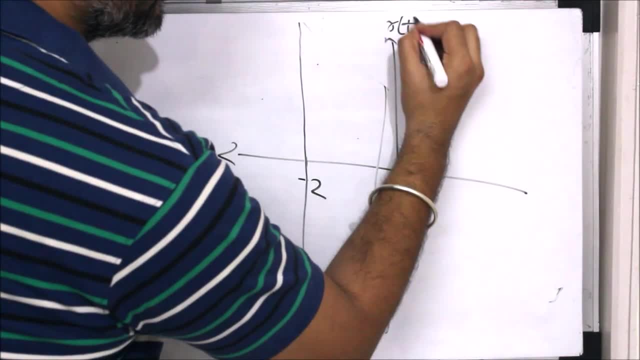 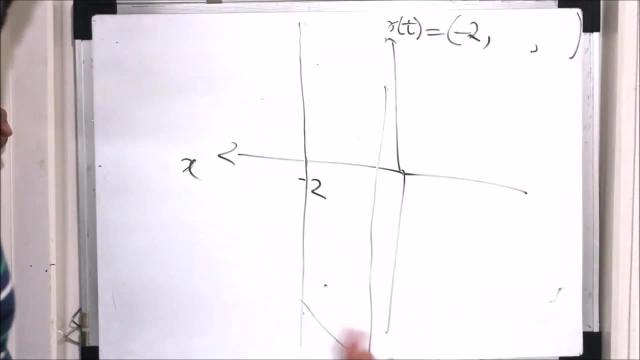 So my what? What will be parameterization? My R of t will be what My x equal to minus 2 is fixed And depending upon the radius and the center. Suppose if I keep the same center, 0 comma 0.. 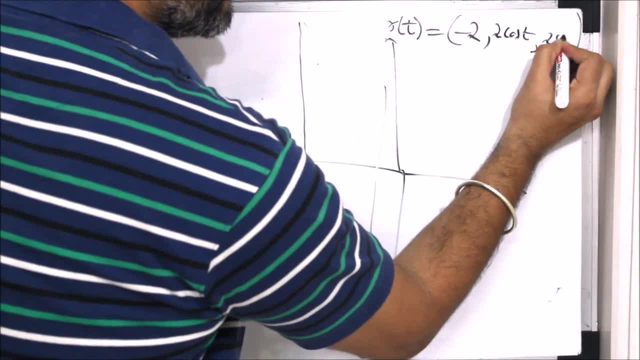 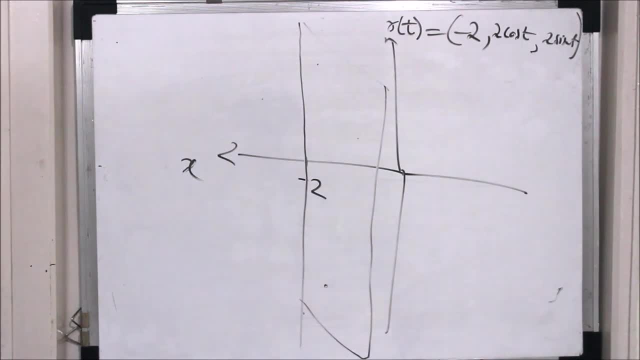 And radius has 2.. So 2 cos t, comma 2 sin t. So this is a parameterization of a circle Which is in which plane Which is, in x, equal to minus 2.. So this is a plane over here. 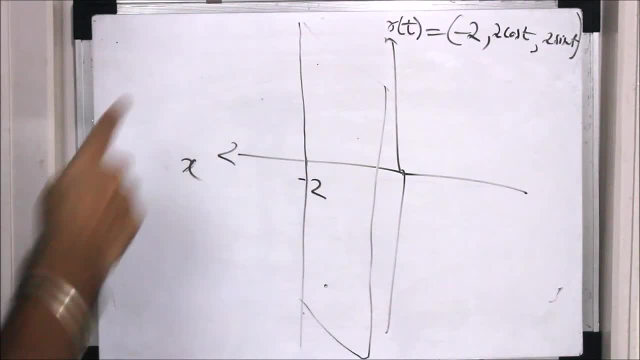 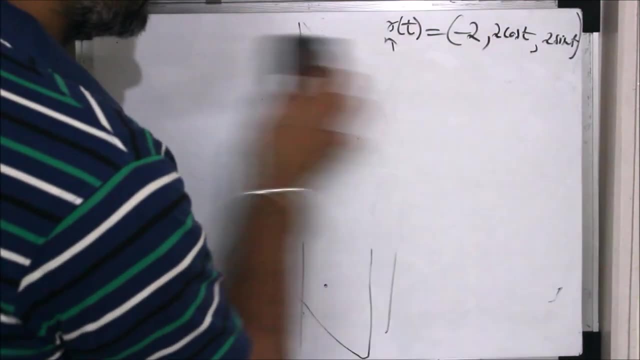 And it is a circle in this plane. So since x equal to minus 2 was fixed, So this is a circle in x equal to minus 2 plane. So that's how you parameterize the curve. You can try to parameterize the curve. 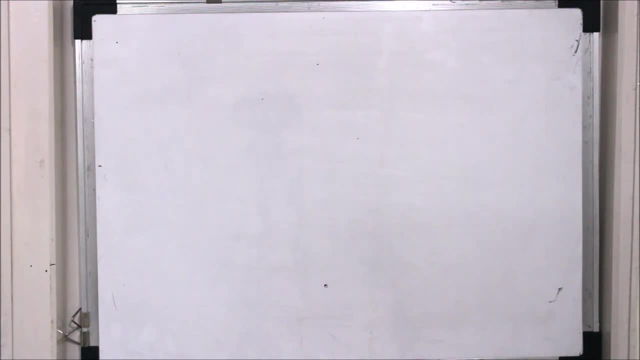 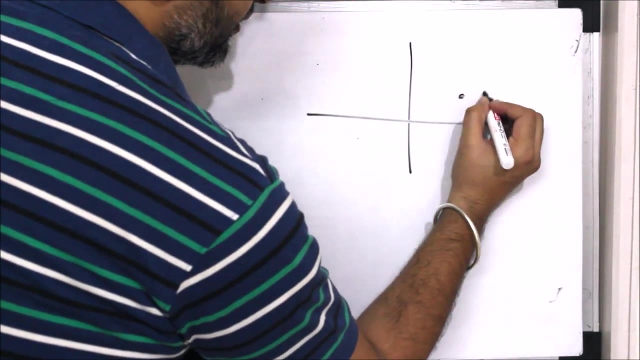 Which is, in say y, equal to 3 plane, And then you take whatever center or radius you want. So that's one thing. Suppose the center is not 0: 0.. Suppose the center is 2 comma 3.. And radius is what? 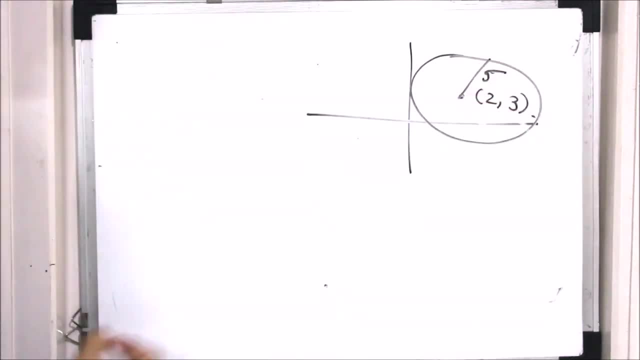 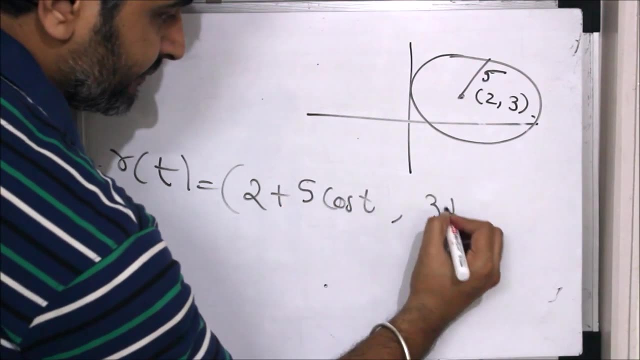 Radius is 5.. So what will be my parameterization? It will be what 2 plus 5 cos t comma 3 plus sin 5 t. Previously the center was 0, 0.. Now the center is what 2 comma 3.. 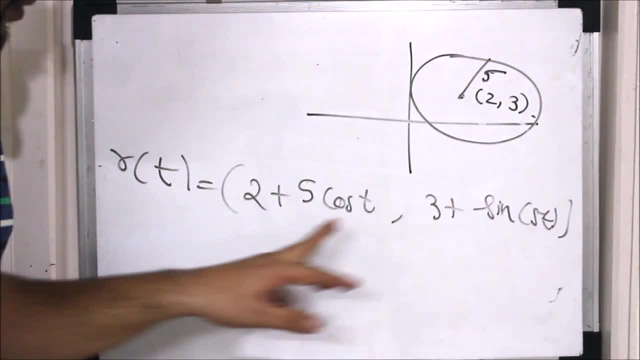 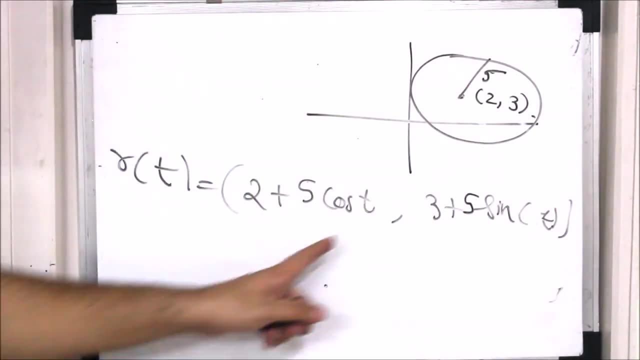 So circle is translated over there. So you simply add 2 and 3. So this will act as the center: 2 comma 3. And this was our normal parameterization of a circle. So if the center is not 0 comma 0.. 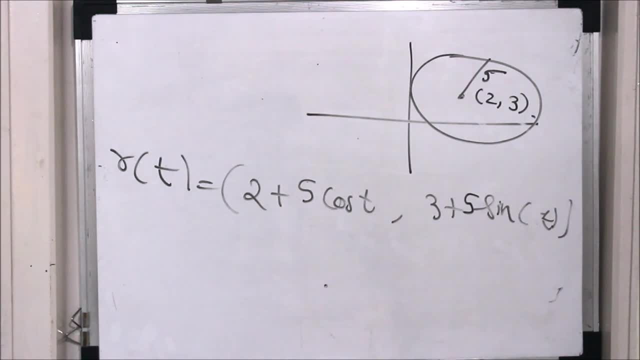 It is something else. Then you add that, For example, 2 and 3. Before the 5 cos t and 5 sin t. So this is a parameterization of a circle With center 2, comma 3 and radius 5.. 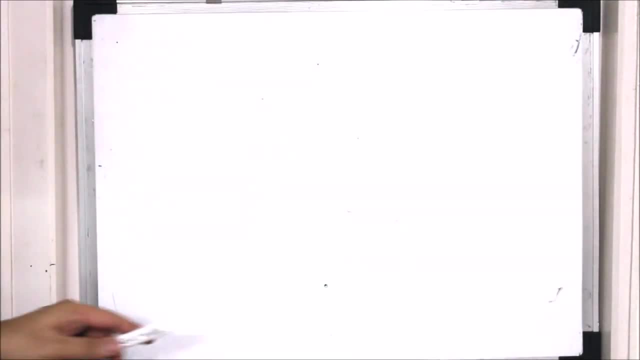 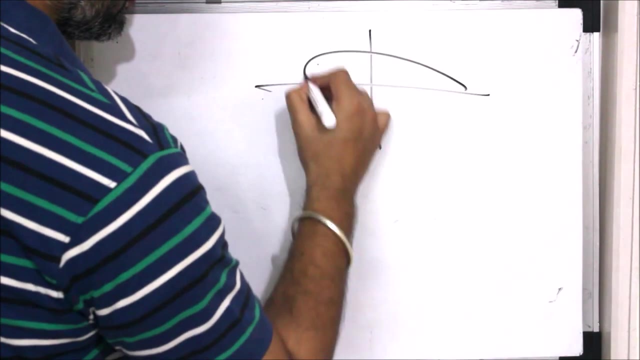 So that's about the circle. If I want to parameterize an ellipse, So if you have an ellipse, Suppose this is 3 and this is 2.. So what will be my parameterization? R of t will be 3, cos t, comma 2, sin t. 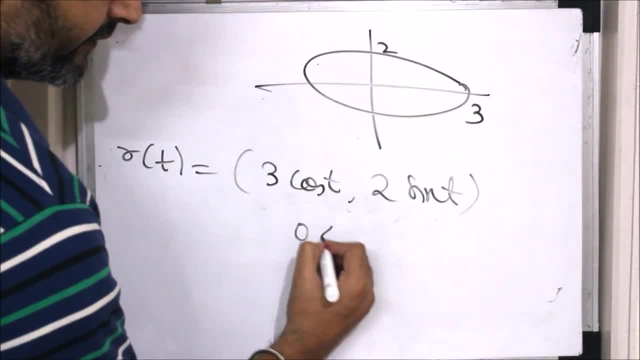 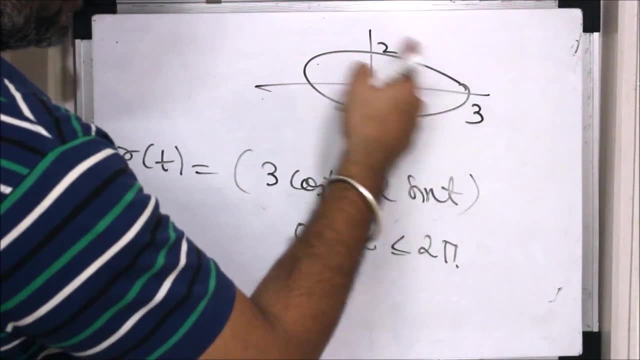 And my t is going from 0 to 2 pi. So as you start from 0 it is at here And as you travel till 2 pi you get whole part of the ellipse. So as you can see in the circle the radius was fixed. 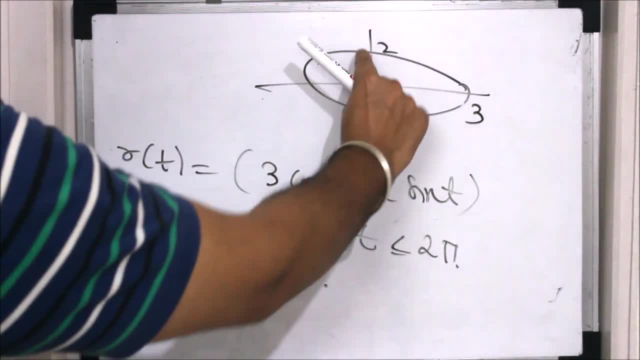 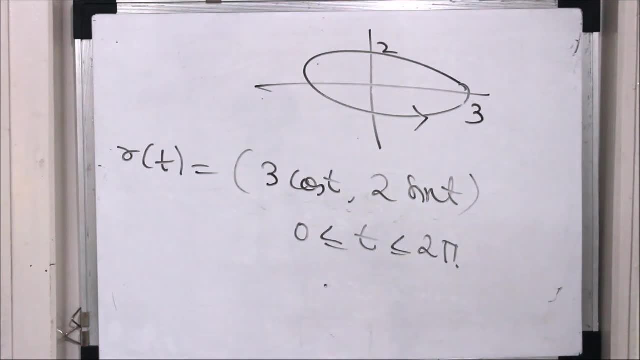 So both these numbers were fixed Here. the major and minor axis are there. Therefore this will be 3 and that will be 2.. So this is a parameterization of an ellipse, And then you can change If you change the range of t. 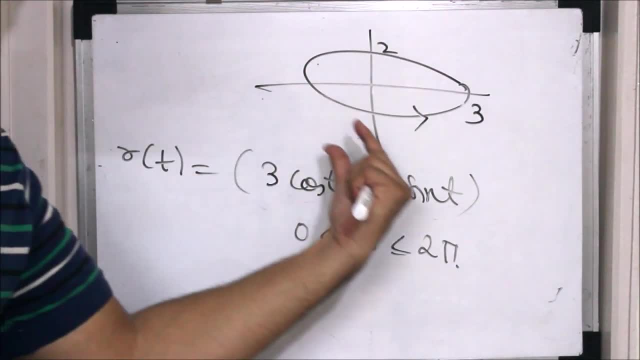 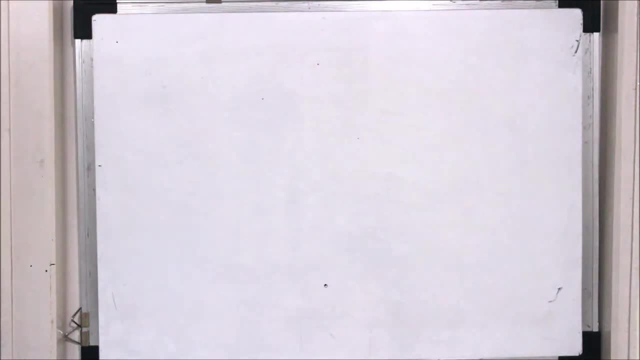 If you change this range of t, You get the specific arc of an ellipse. So that is how you parameterize an ellipse. What are the other standard curves you have seen? Okay, let's go for parabola, Suppose, if you take parabola, 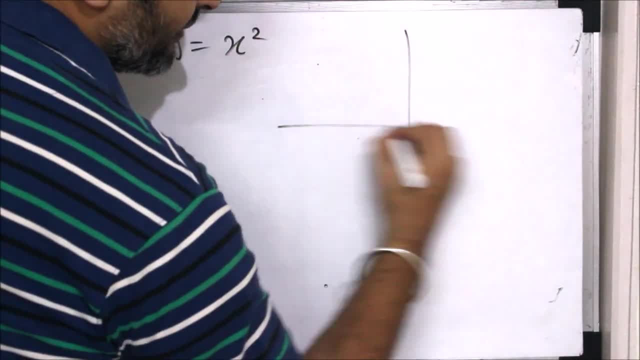 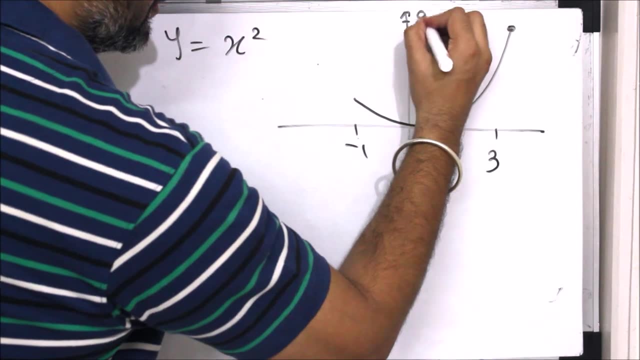 Suppose you have y equal to x square And I want to parameterize: only say this is minus 1 and this is say 3.. So this is a parabola and I want to parameterize it. So how will I parameterize? 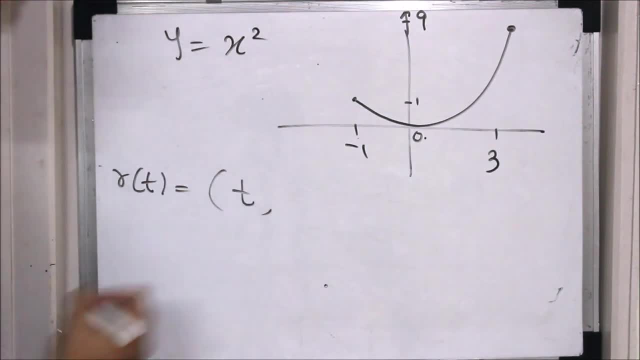 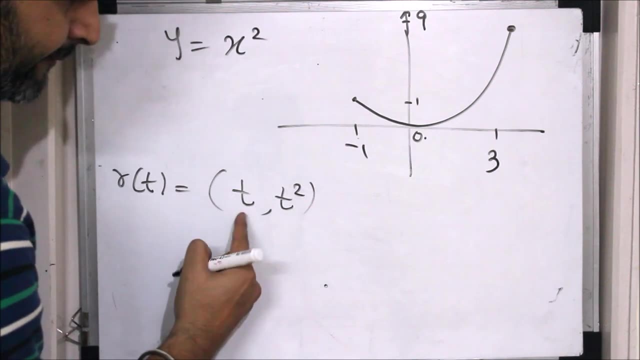 R of t will be what If I put x equal to t? what will be my y? If you look here, my y will be nothing but t square And my x was t. and my x is going from where to where. It is going from minus 1 to 3.. 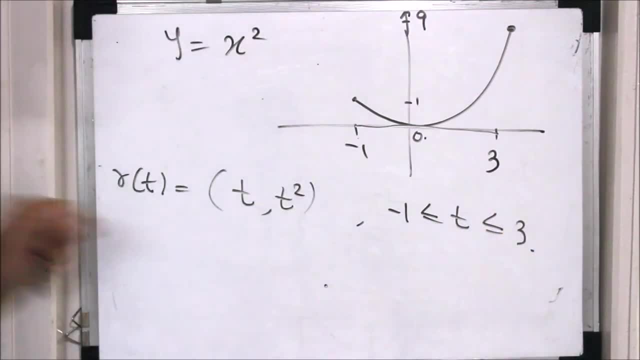 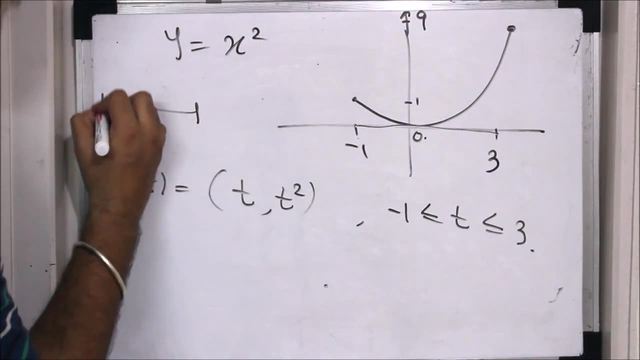 So minus 1 less equal t less equal 3.. So this is a parameterization of this parabola And, as you can see, my t is minus 1.. What is the image of minus 1?? Minus 1 will go to minus 1 comma 1.. 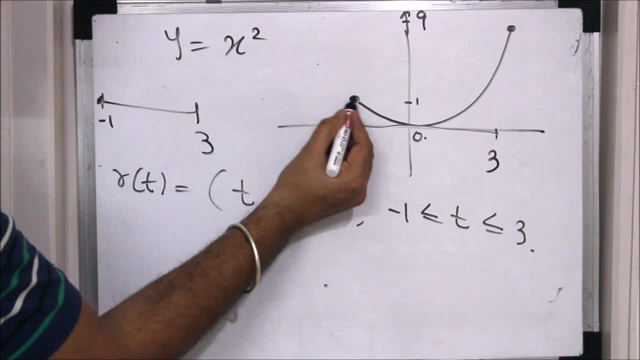 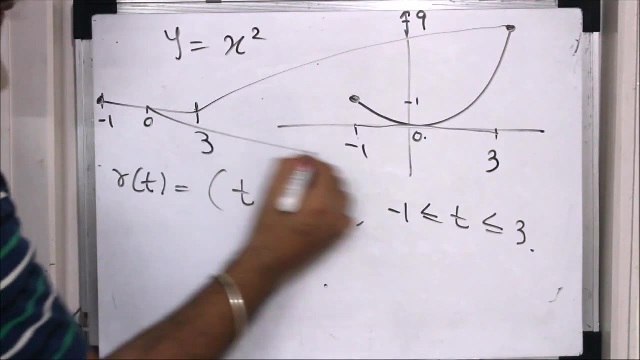 So this point, This point will go to this point. What is the image of 3? 3 comma 9.. So this will go to where? Here, Where my 0 will go, 0 will go to 0 comma 0.. 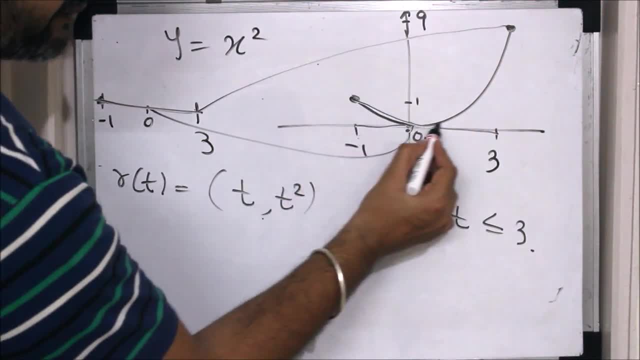 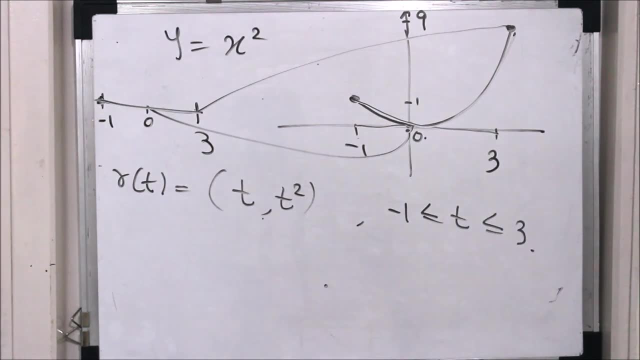 So as you go from minus 1 to 3, you are covering all the points on this curve. So image of R is nothing but the parabola. So that is how you can. So usually whenever some equation is given to you, 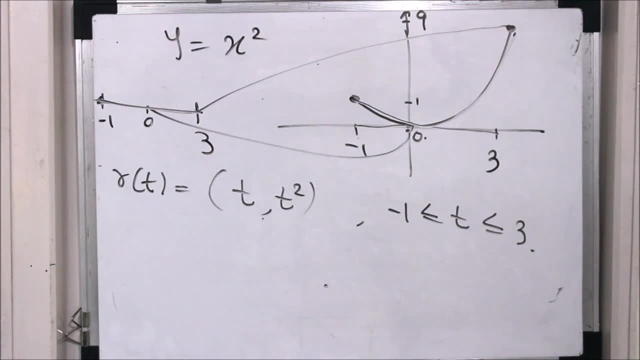 You put x equal to t or y equal to t or whatever, z equal to t And, depending upon the equation, You put the value of x equal to t and then you get the remaining substitution for y and z. So that's how one do the parameterization. 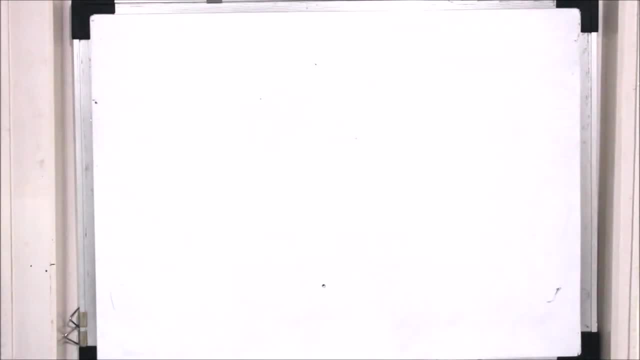 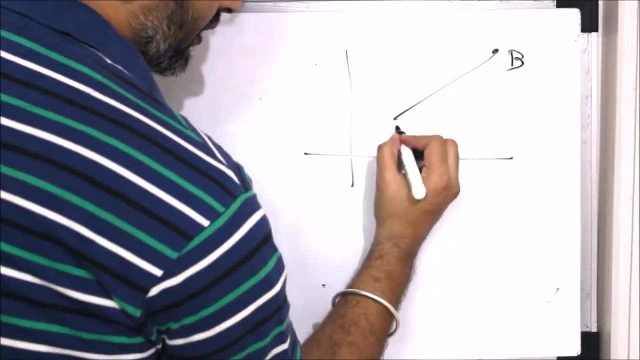 So there is one thing. Suppose I want to parameterize a line. If I want to parameterize a line, So I have a line joining the point a and b. So what I will do is I will take domain as 0 to 1.. 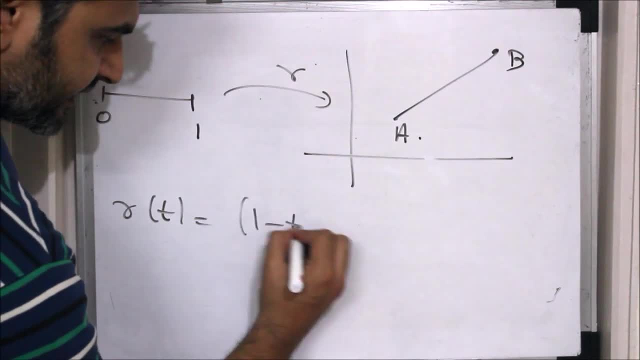 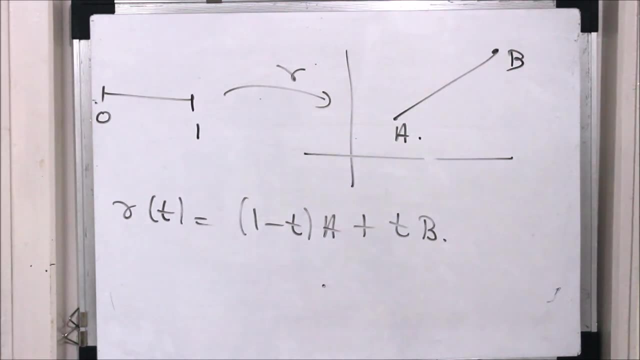 What R of t I will take. I will take 1 minus t into a. This is the standard parameterization of a line. Most of you might have seen this when they have studied vector equations. So, as you can see, when my t is 0.. 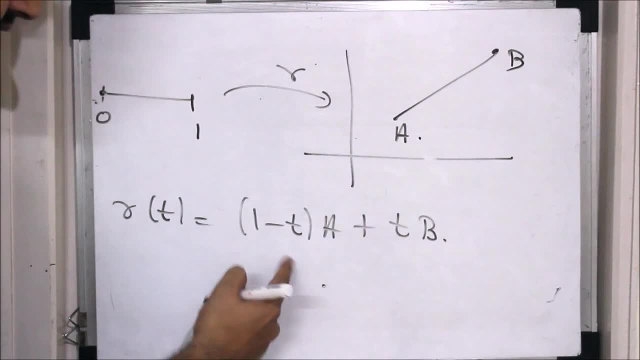 When my t is 0. This is what a plus 0 b. That means a. So that means image of 0 is what a? That is the starting point of the line When my t is 1.. This is what. 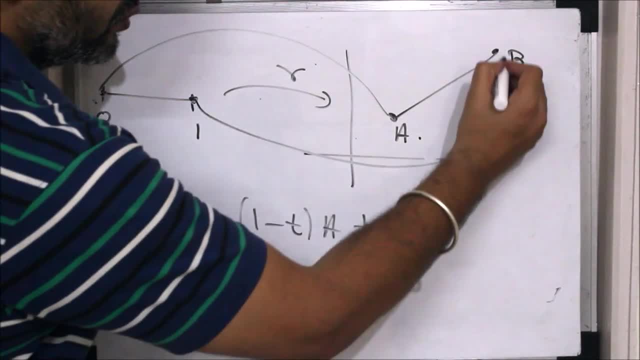 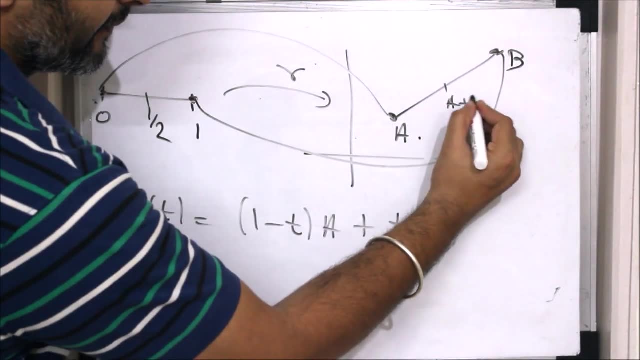 1 minus 1. This becomes 0. This is 1.. So this becomes So 1 is going to b If I take 1 by 2.. This is a plus b by 2.. So this will go to the midpoint. 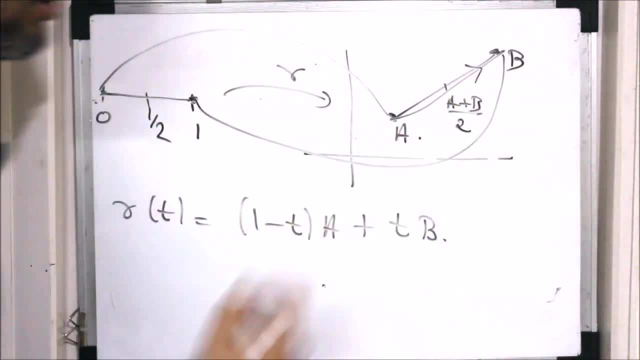 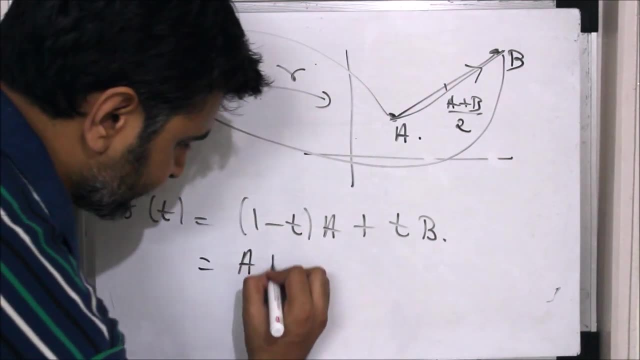 So, as you go from 0 to 1. I am getting all the points on the line a to b. So this is what the parameterization of a line is. Another way of writing this is nothing but a plus b minus a, including. 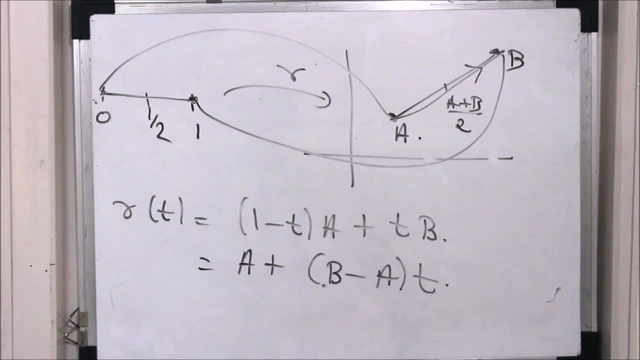 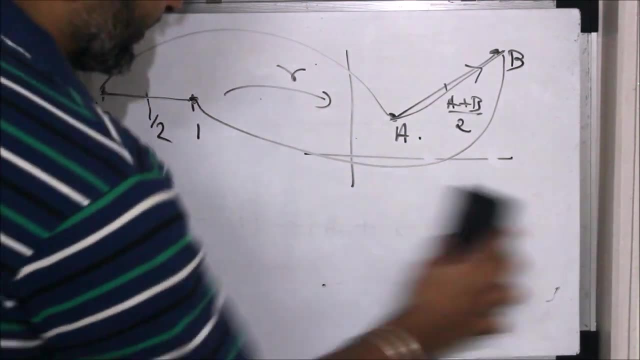 Where t is from 0 to 1.. So this is the standard parameterization of a segment Which we will be using more frequently. So this is one thing. Let's take an example. Suppose I want to parameterize a line joining. 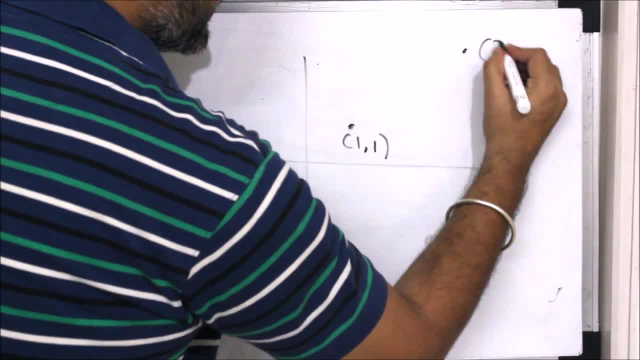 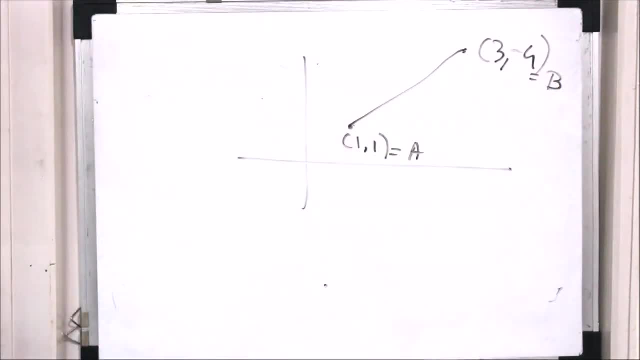 So this is say 1 comma 1.. And say this is 3 comma 4.. I want to parameterize this. So what is my a a is this And what is my b? point b is 3 comma 4.. 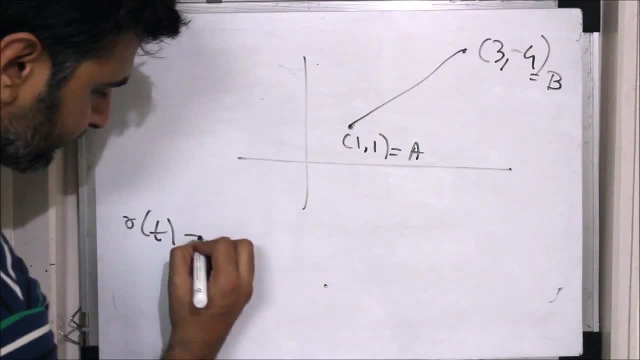 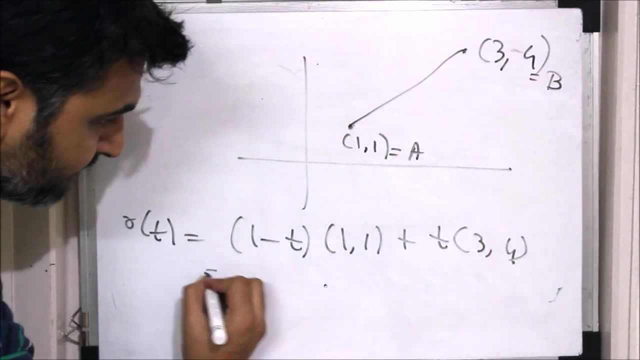 So what is the parameterization? r of t is nothing but 1 minus p into a, Which is 1 comma 1. Plus p into b, Which is 3 comma 4.. If I simply multiply this, This is 1 minus p, comma 4.. 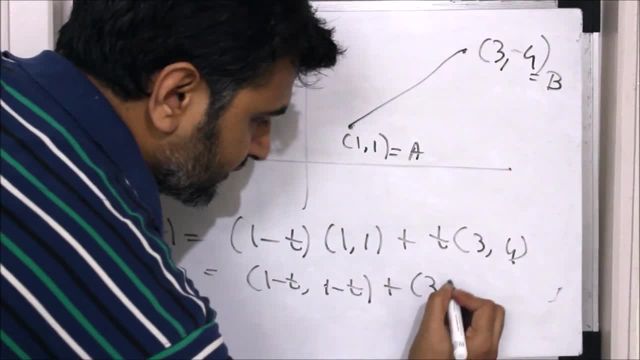 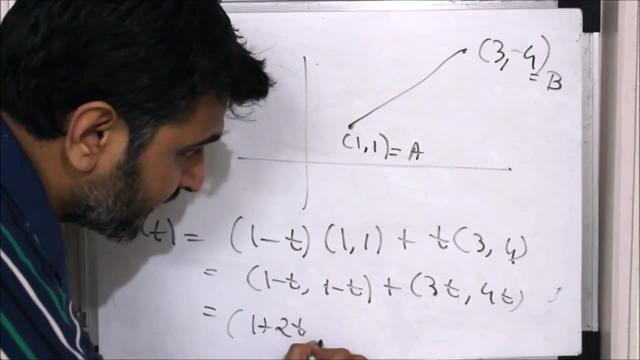 1 minus t comma 1 minus t Plus 3t comma 4t, And if I add them It is nothing but 1 minus t plus 3t is nothing but 1 plus 2t, And this is 1 plus 3t. 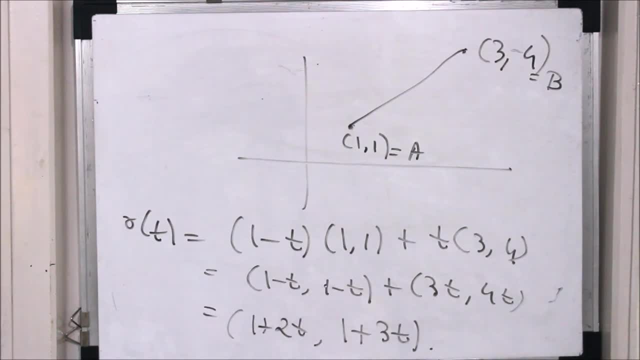 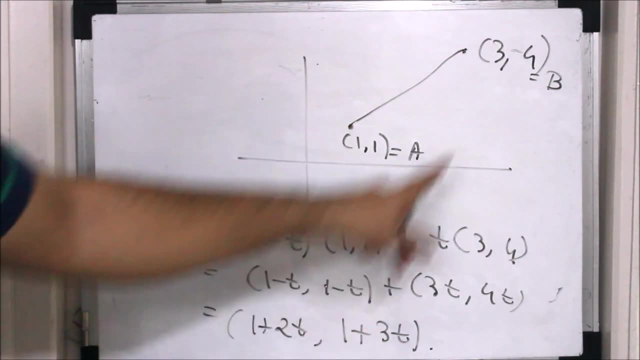 Where t is going from 0 to 1.. So this is the parameterization of this segment. As you can see, when my t is 0. I am getting 1 comma 1.. When my t is 1. I am getting 3 comma 4.. 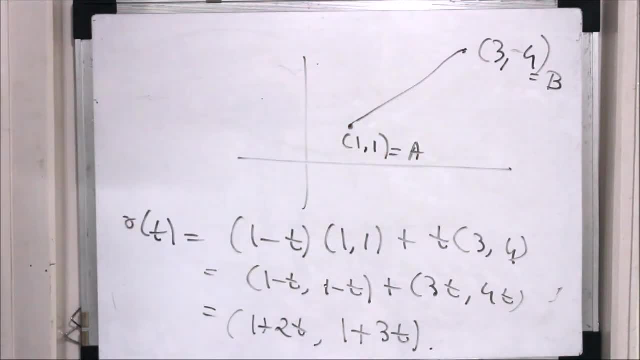 And as you go from 0 to 1.. All the points on this circle. Okay, So that's one thing. So that's how we parameterize a segment. So we are done with the circle. ellipse parabola line segment. 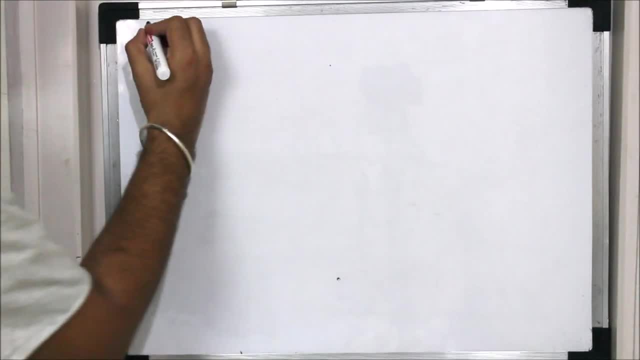 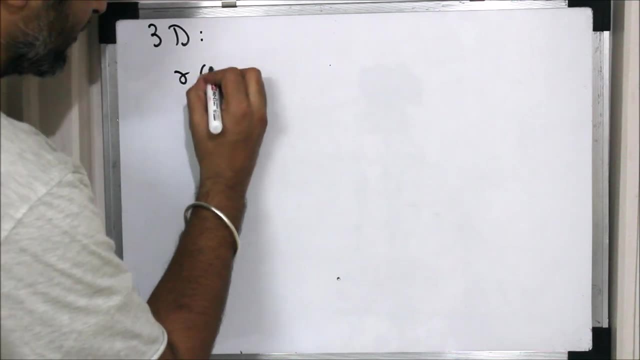 Okay now. So let's go for the 3D curves. So if you have a curve in a 3 dimensional space, So say, for example, If I take r of t as Plus p comma, sin t. Now if I close the bracket here, 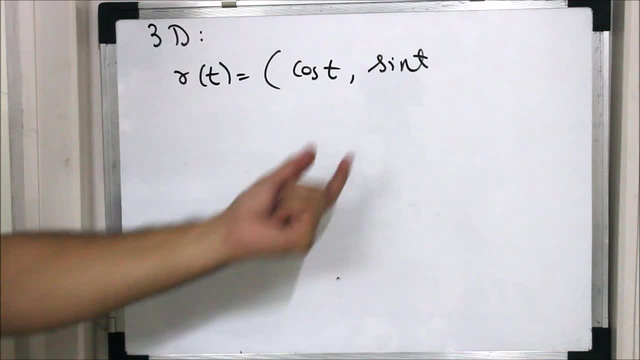 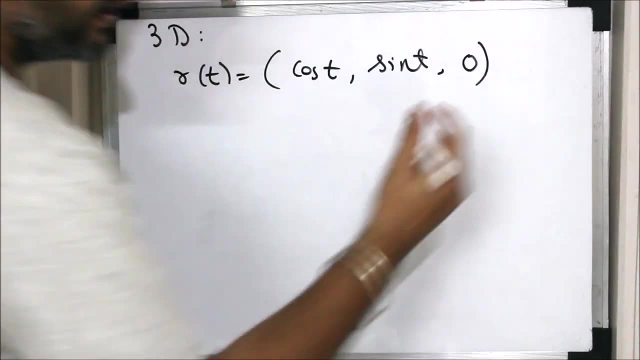 This is nothing but a circle in my circle. This is nothing but a circle in my 2 dimensional space. This is a circle in xy plane With center 0 comma 0 and radius 1 comma 1.. And suppose, if I mention that, 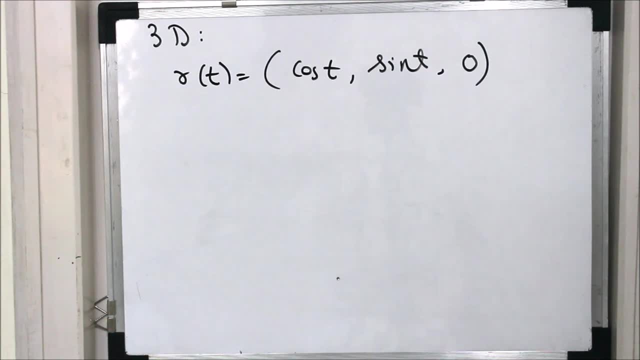 If I want to mention that, Look at this curve In r3.. But in the xy plane, Then what I will do, I will introduce a z component. I will put that as 0.. But suppose, if I want to say: 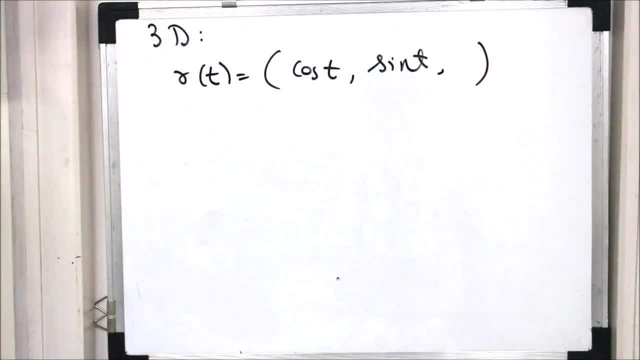 Consider a circle in z equal to 1 plane. If I want to say, Consider a circle in z equal to 1 plane, So I will fix my z equal to 1.. As this is a circle, So this is again a circle. 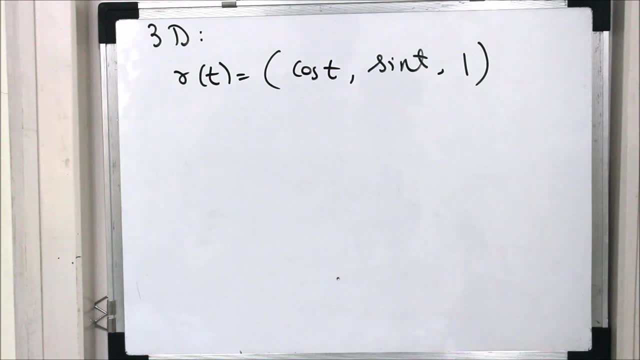 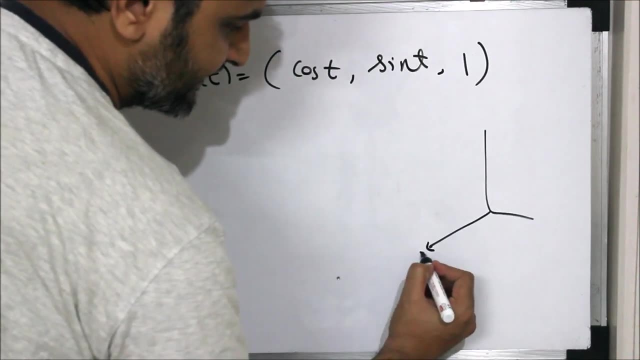 But instead of looking into xy plane, We will look at z, equal to 1 plane. But now suppose, Like, whatever, So this is nothing. but If this is my x And this is my y And this is my z, 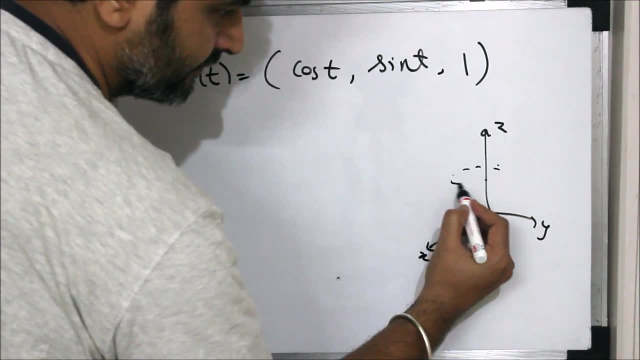 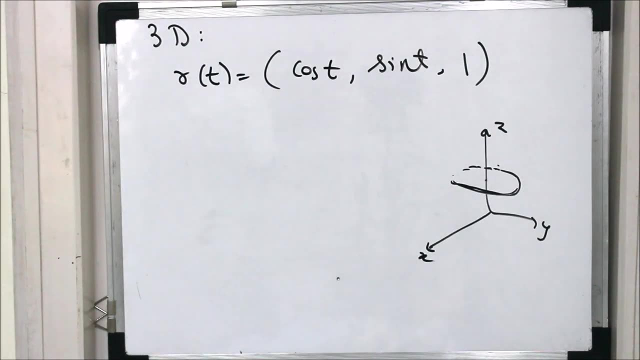 This is a circle Here in xy plane, So it's a circle in. Sorry, It's a circle in z equal to 1 plane. So this is the circle in z equal to 1 plane. But now suppose, Instead of fixing this z component. 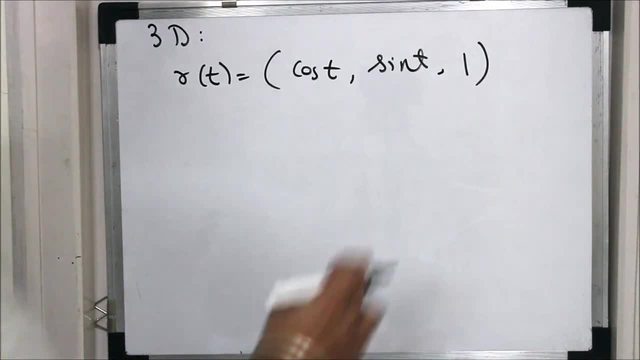 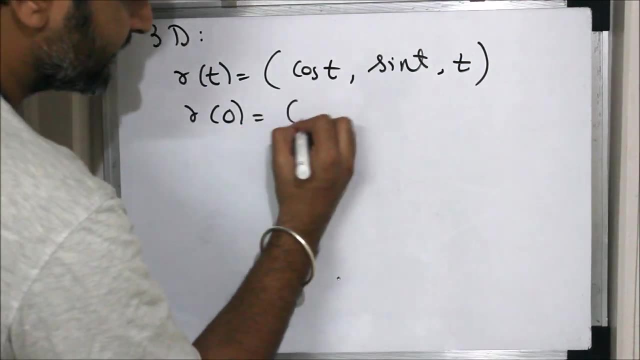 Let me vary this z as well. So if I vary this z as well, Suppose, let's take this as t. Okay, Now you see what will happen When my t is 0.. What is r of 0?? It is 1 comma 0 comma 0.. 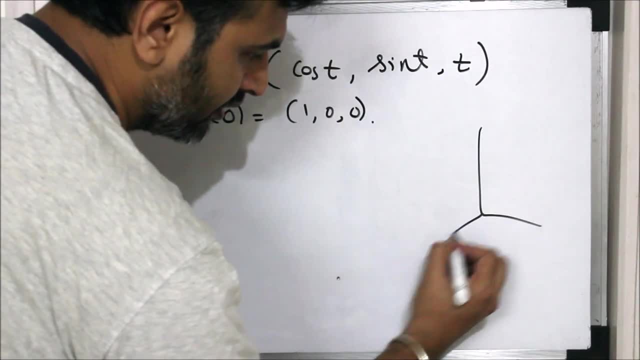 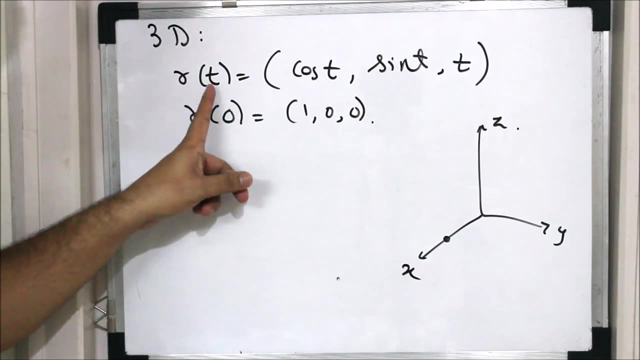 So it is nothing, but It's a point in. It's a point on x axis: 1 comma 0 comma 0.. Now, as my t will increase, This point will no more Be in xy plane Because, as my t will increase, 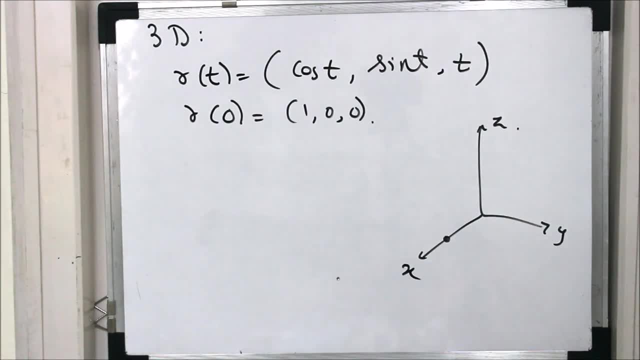 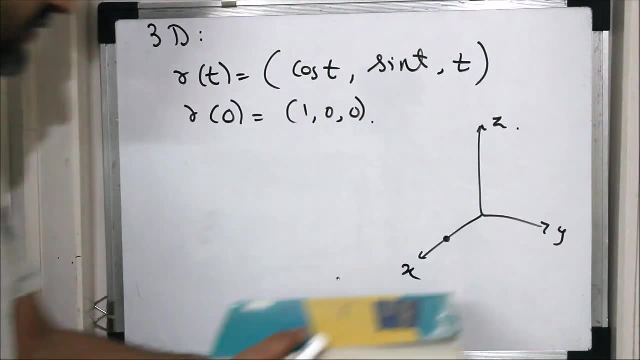 My third component will also increase And because of this, what will happen is I won't get a point in xy plane. So if you say I mean, if this is my xy axis, I mean what you can do is Yeah. 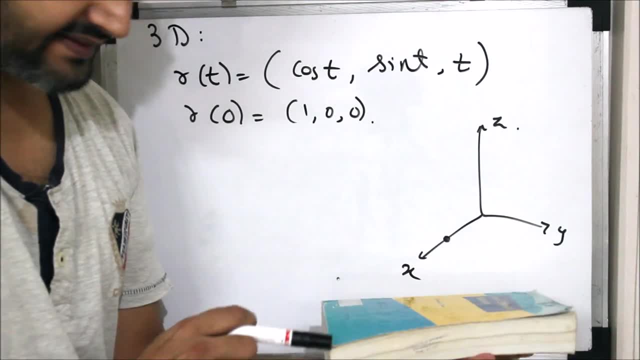 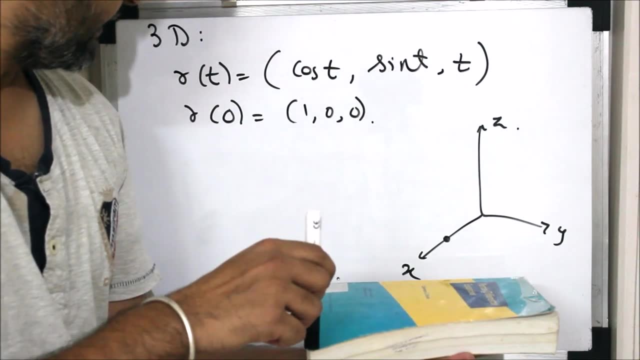 This is my x axis, This is my y axis And this is my z axis. So x axis, y axis and z axis. So when my, When my t was 0, I was getting this point 1 0, 0.. 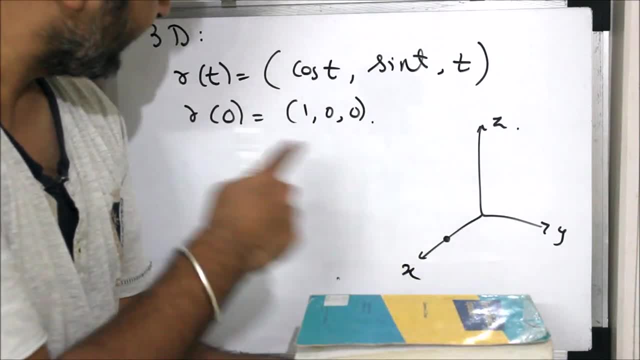 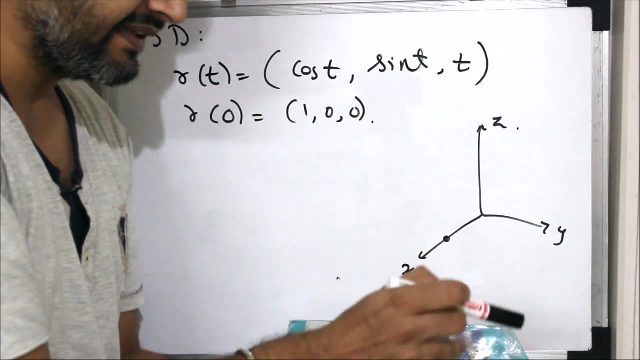 So on the x axis this point is 1 comma 0 comma 0. Now, as my t will increase, Previously it was 0. So I was getting a circle in xy plane, But now, as my t will increase, The next point won't be in xy plane. 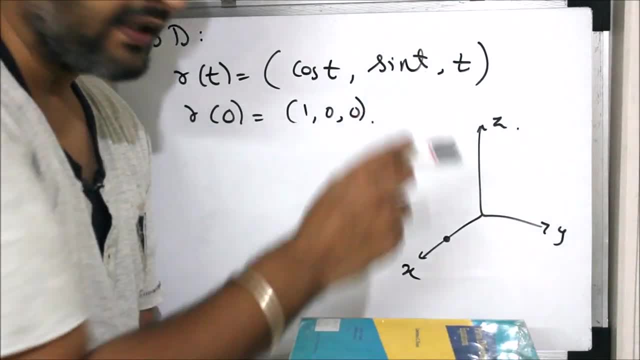 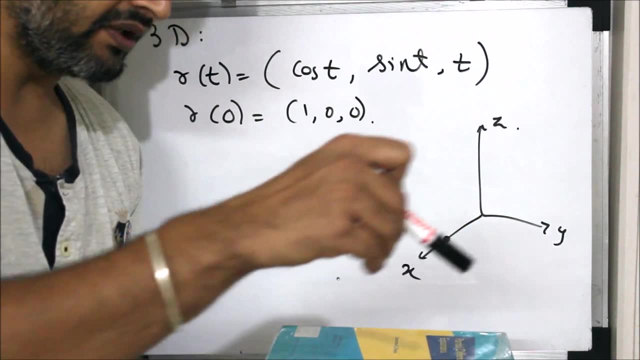 It will be. It will be above xy plane Because the height has increased. So now, as my t will increase, instead of getting a circle over here, What I will get is this circle: The curve will keep on increasing. the curve will keep on increasing by though I'm getting a circle, no doubt, but then it's. 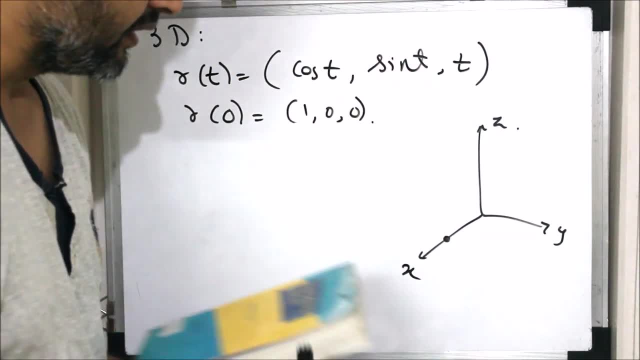 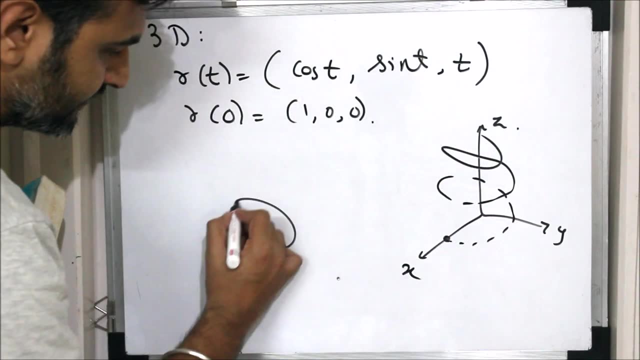 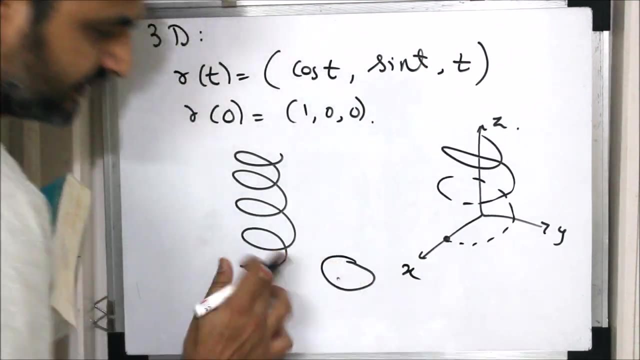 not a circle, it's a kind of a spring you can imagine. so I'm getting a spring. so what I'm saying is like this: I'm getting a spring like this, of fixed radius, one. when I collapse, this, if I keep this zero, if I collapse, what I get I get a circle. so this is nothing, but it is. 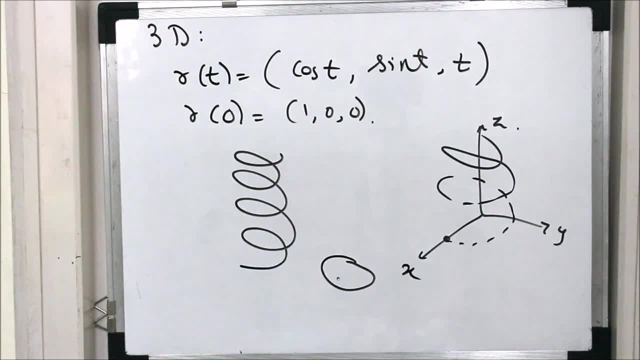 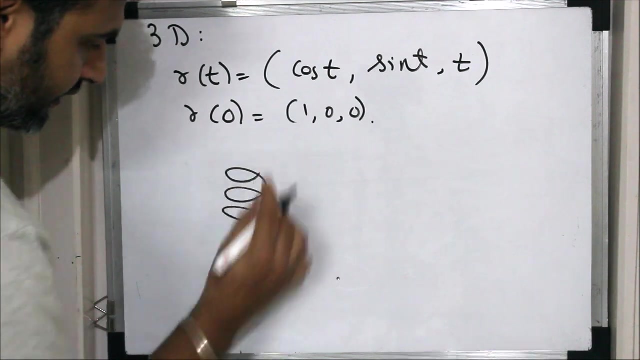 called as helix, or you can say spring. so therefore this is a parametrization of a helix. so that's one thing. okay, suppose, if I don't want to fix the radius of the helix, so right now I was getting a circle, means I was getting this helix right here. the circle radius was fixed. 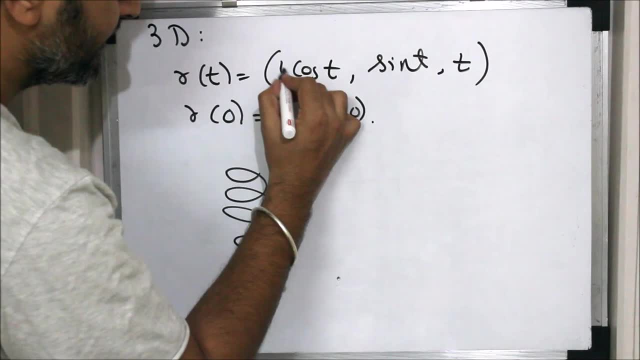 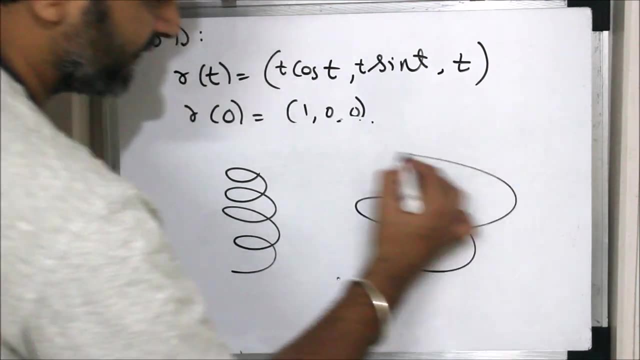 but if I want to increase the radius as well. so what I will do is I will make here t and and t. so what this will happen, what this will make, even my radius is also increasing. so what i'll get, i will get, like this, of helix, so i'll get bigger, bigger radius, because as my t is increasing, 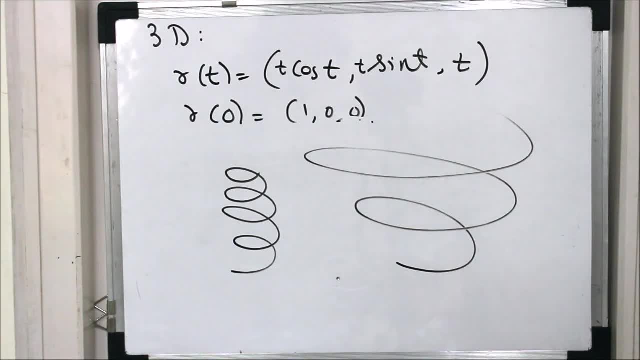 my radius is also increasing. so this is how the helix looks like and one can modify this. if i k times t. if my k is less than one, the radius will keep on decreasing. if my k is bigger than one, radius will- i mean the height will- increase very drastically if my k is less than one. 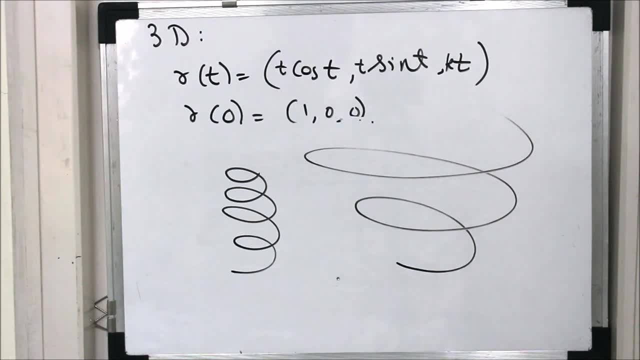 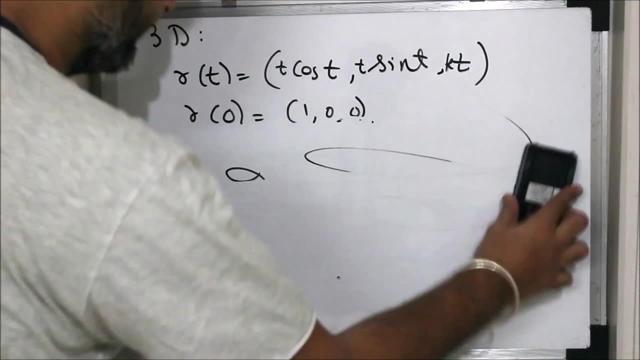 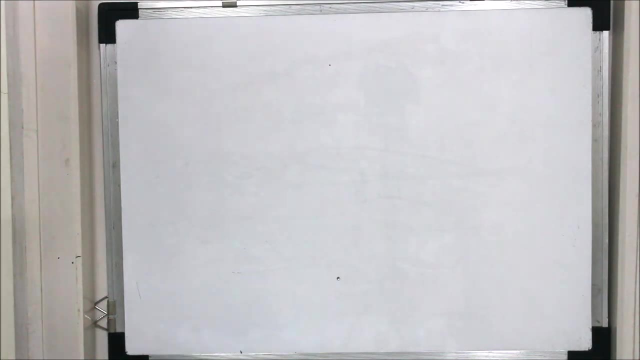 height will increase little bit slowly. ultimately you get all different kinds of spring. so this is a parameterization of a helix. uh, let's go the reverse way, suppose. suppose, if you know the parameterization, how to obtain the equation of a curve in cartesian coordinates? suppose, if i give you r of t equal to say 0, comma t, comma t, square. 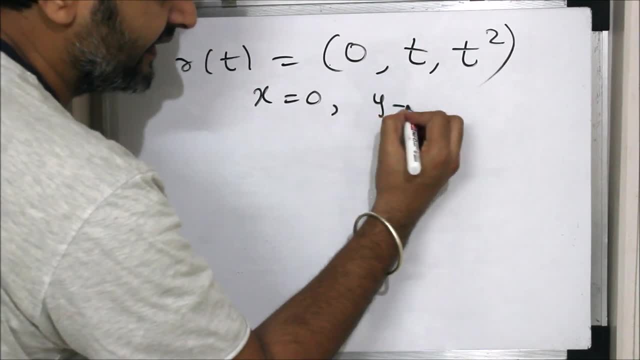 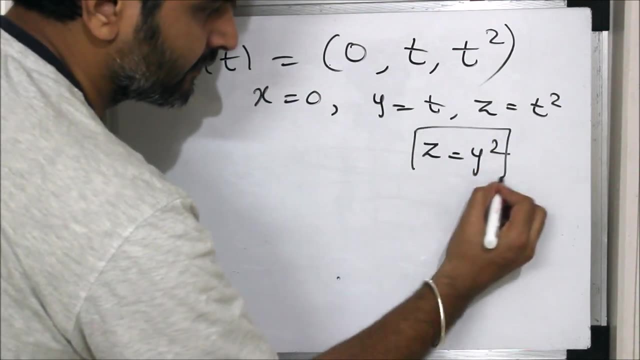 that means? for what is this? this implies my x is 0, my y is t and z equal to t square. and from this two equation what i can see, my z is what y square and my x is what 0. so in x equal to 0, plane means which? 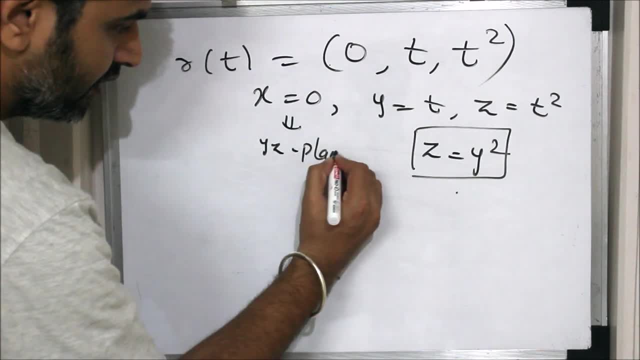 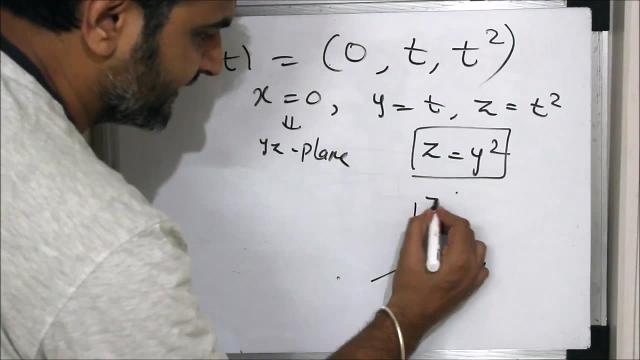 means which this is nothing but my y z plane. so if i look into y z plane, i am having a parabola. so this is my y z plane, y and z plane. in this plane i am having a z equal to y squared parabola. 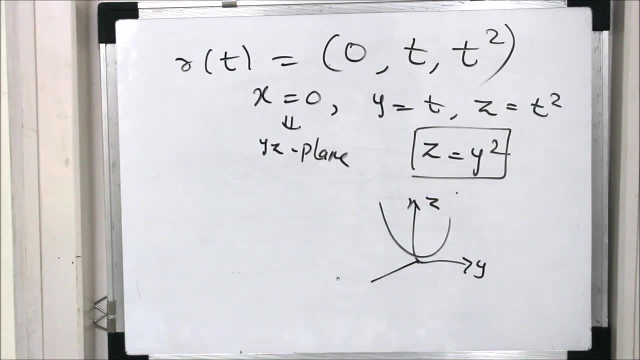 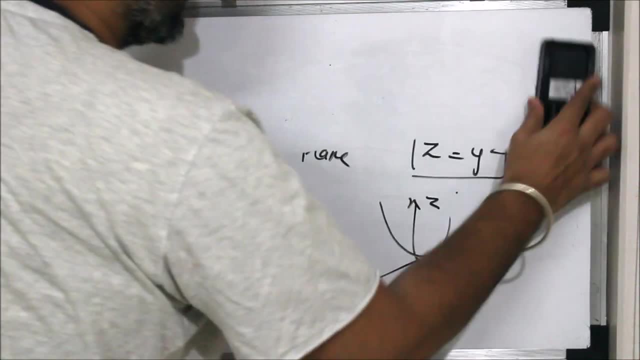 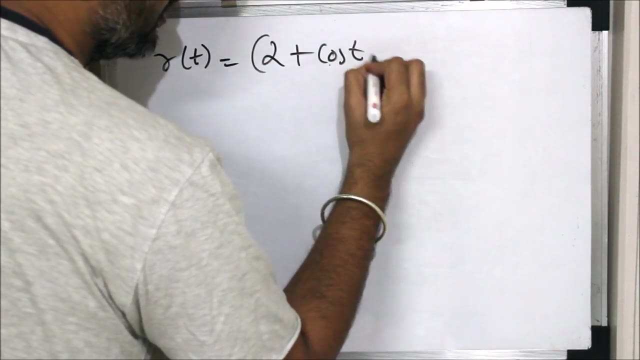 because first対 państwo. so once you have a parameterization you try to eliminate p by bringing into xyz into the picture. so if i take one more example, suppose if i take r of t equal to 2 plus cos fie, 7 plus sine t, and if i take 3, that means what i am, in which plane i? 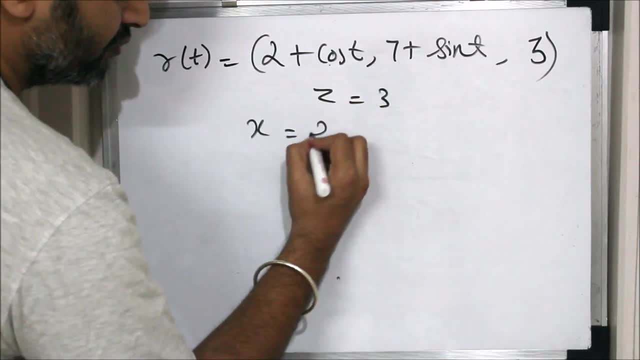 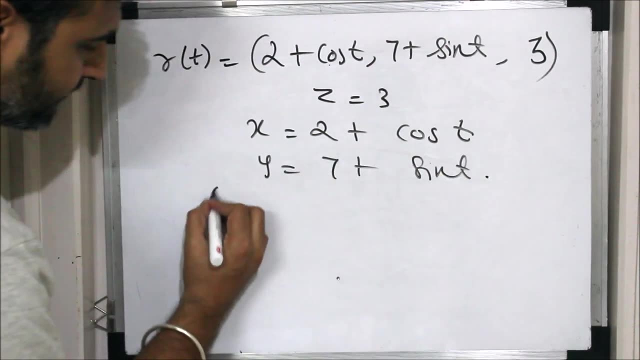 mean z equal to three plane. and what is this? x equal to two plus cos fiel. and what is this? x equal to two plus cos fie, one plus sine t. and what is this? 3? what is this? y equal to 7 plus sine t. so this is nothing but x minus 2 square plus y minus 7 square. 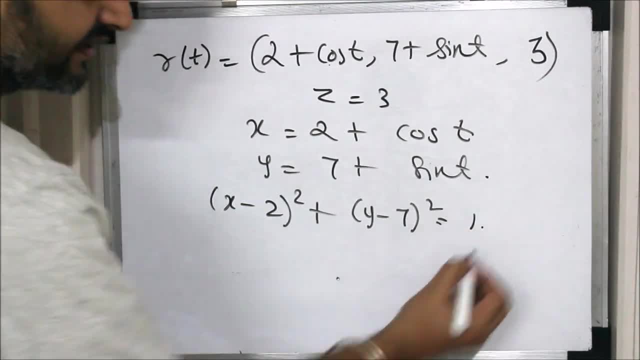 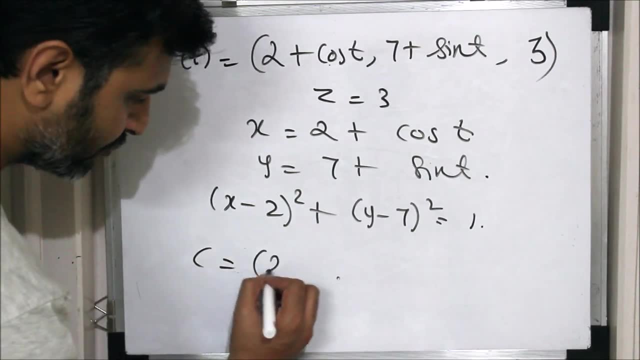 x minus 2 is what cos t? so cos square t plus sine square t is nothing but 1. so what is this? this is nothing but a circle with center 2 comma 7. so in this case my center will be 2 comma 7, my radius: